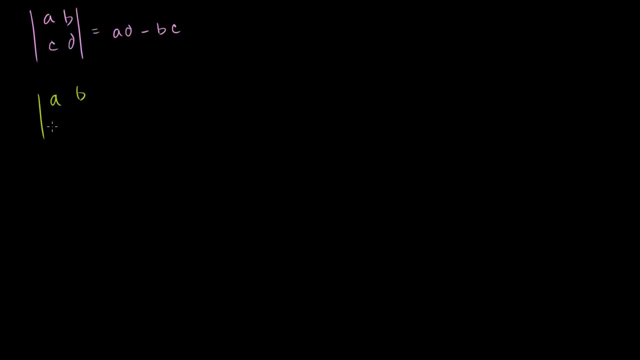 So we have the situation a- b. Let's multiply the second row times k. So we have k c and k d. Now what's the determinant going to look like? We're going to have a times k d, or we could just write that: 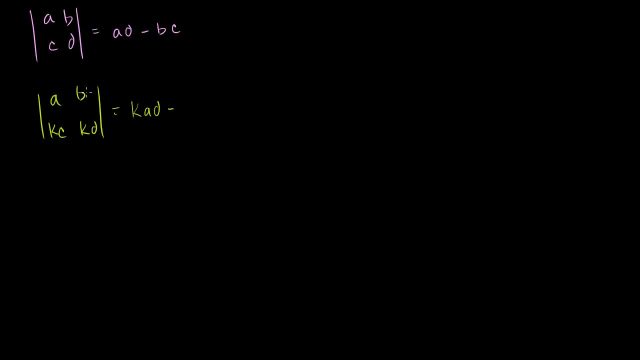 as k a d minus k c times b. or we could write that as k b c. If we factor out the k, we get that equals k times a d minus b b c. Now you immediately see that this thing is the same thing. 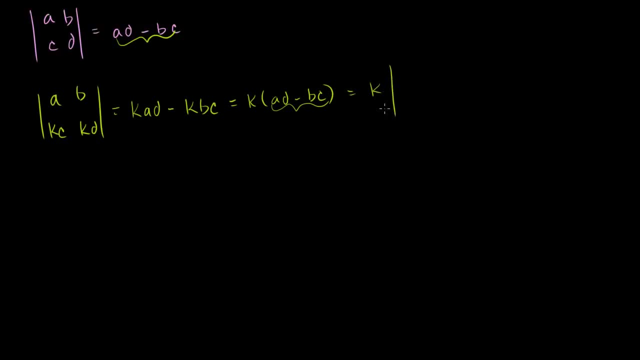 as this thing. So this is equal to k times the determinant of a, b, c, d. So when you just multiply a row by a scalar, just one row, not the entire matrix. when you just multiply a row by some scalar, the resulting determinant will be the. 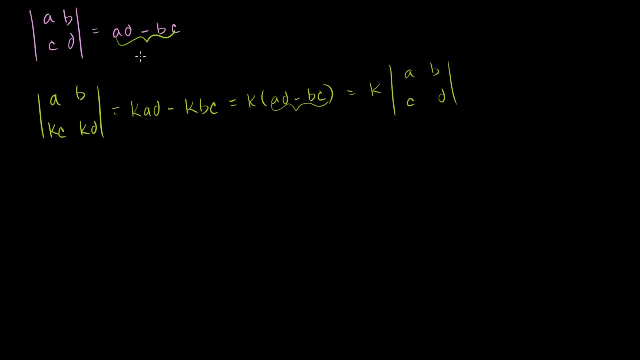 original determinant times that scalar. Now you might say: well, what happens if I multiply the whole matrix times that scalar? Well, that's equivalent to multiplying by a scalar twice, right, If I say that? let's say I have the matrix A and the matrix A. 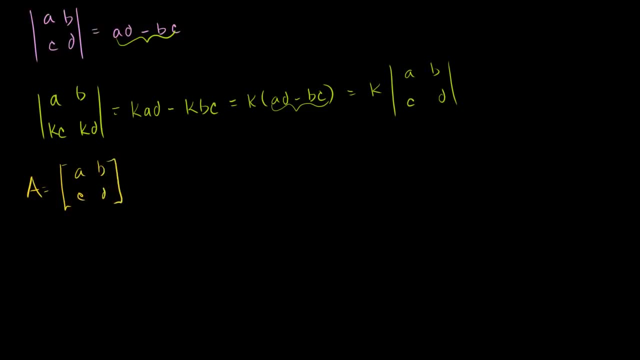 is equal to a, b, c, d. If I were to think about the matrix k, a, now I'm not just multiplying one row, I'm multiplying the whole matrix by a scalar. This is going to be equal to k lowercase a, k, b, k, c and. 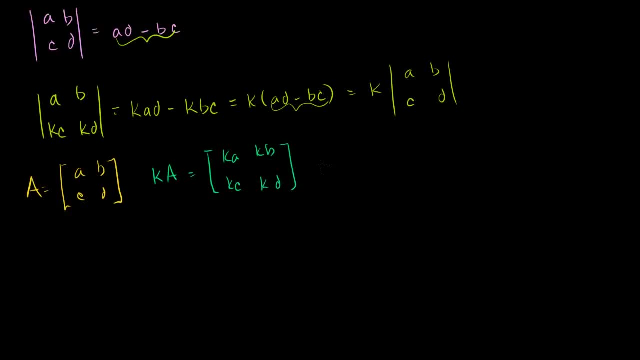 k d And when you figure out its determinant, the determinant of k times a is going to be equal to the determinant of k a, k b, k c and k d. And here you're immediately going to see, you're going to. 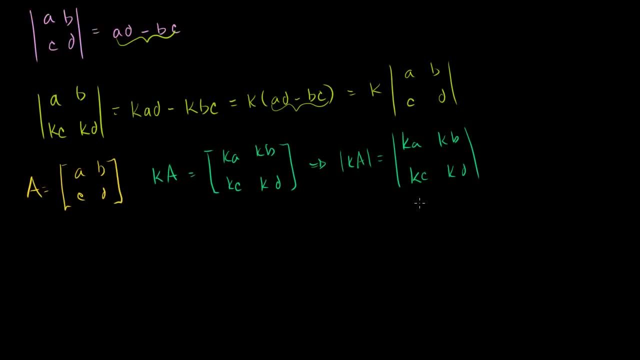 end up with k squared terms. You're going to have k squared times a. d is going to be equal to k squared a, d, minus k squared d- c, Or k squared times a- d is going to be equal to k squared. 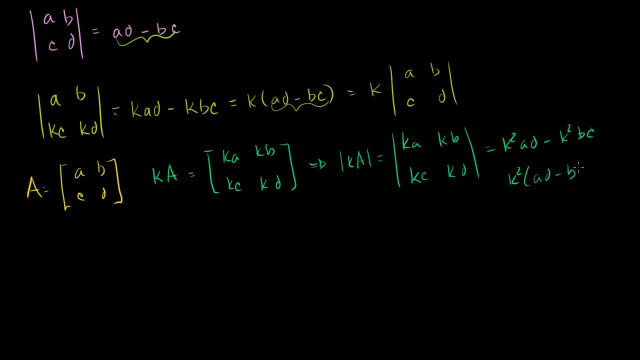 times a, d minus b, c Or k, squared times the determinant of just a. So you have to be very careful, And this is only for a two-by-two case. You'll find out that if this was an n-by-n matrix, that 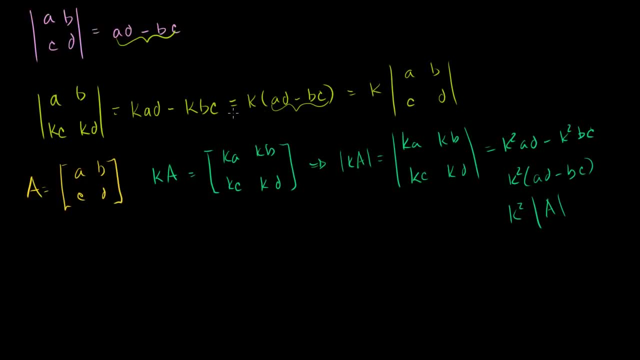 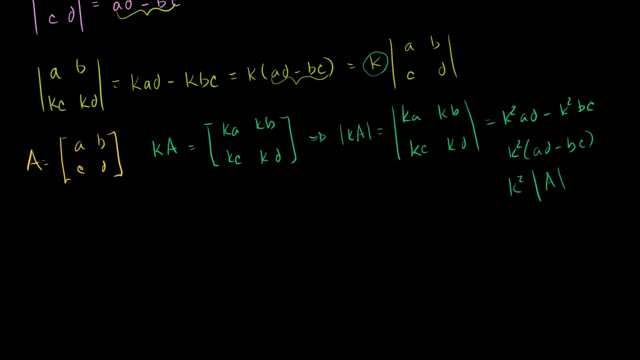 this would have been k to the n. So the takeaway is the only way you can say that it's going to be a sum scalar multiple times your original determinant is only if you multiply one row times that scalar multiple, not the whole matrix. So let's see how this extends to maybe a three-by-three case. 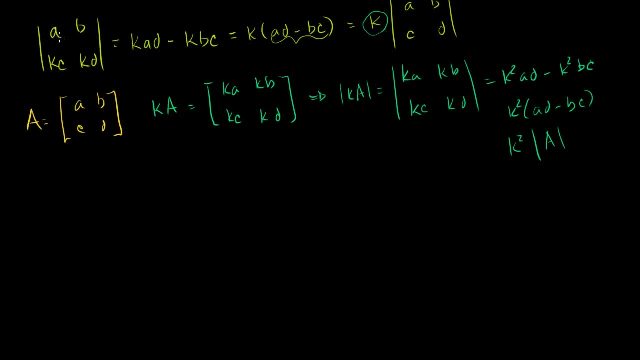 And you might say: hey, Sal, you just picked the second row. it doesn't work with the first row, I'll leave that for you to determine. but it does work. It doesn't matter which row I multiplied it by. Let's take the three-by-three case. 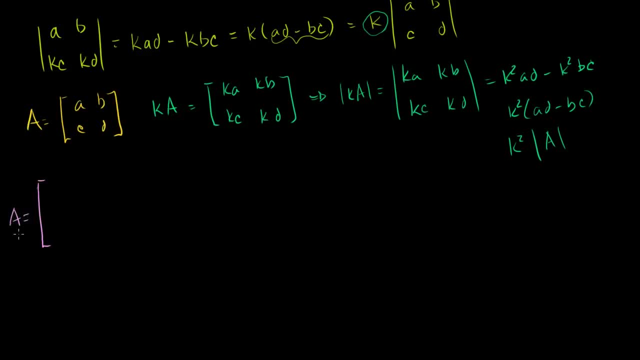 Let's say we have some matrix. Let's call this a again. I'm redefining a. It's going to be a. b, c, d, e, f, g. It's going to be a, b, c, d, e, f, g, h, i. 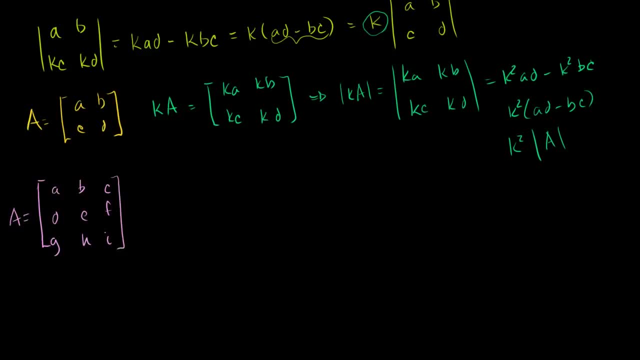 And then, if you take its determinant, the determinant of a is going to be equal to well, we could do it a couple of different ways, but I'll just pick some arbitrary row, because that's the row that we're going to multiply by. 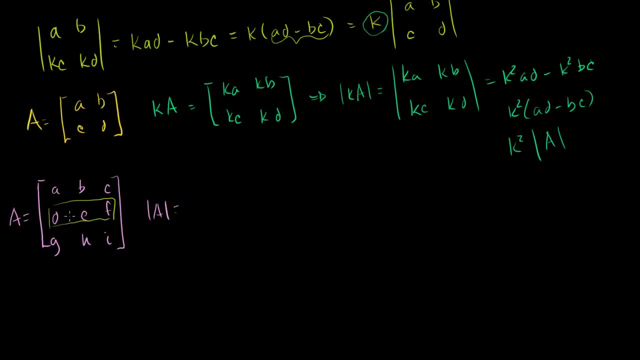 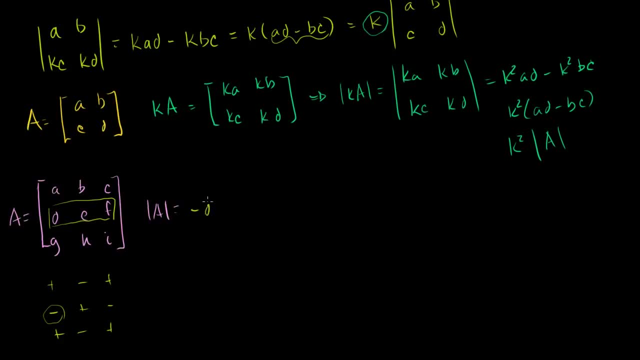 So d is a minus right there. So it's going to be equal to minus d times the determinant of its submatrix. So you cross out that column and that row. It's b, c, h, i and it's going to be plus e times its. 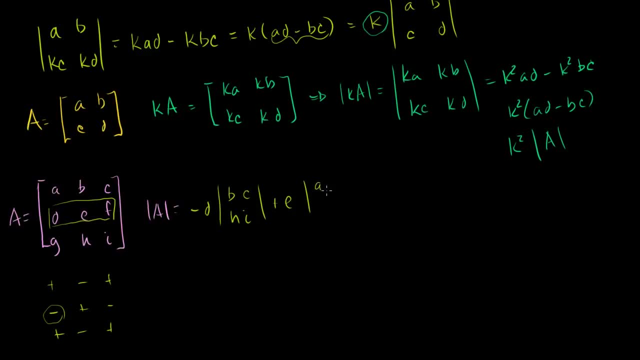 submatrix a, c, g, i, and then it's going to be minus f times. you get rid of that row, that column d e g h, the determinant of d e g i. 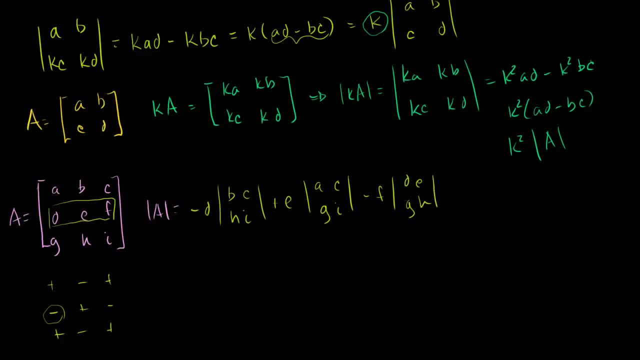 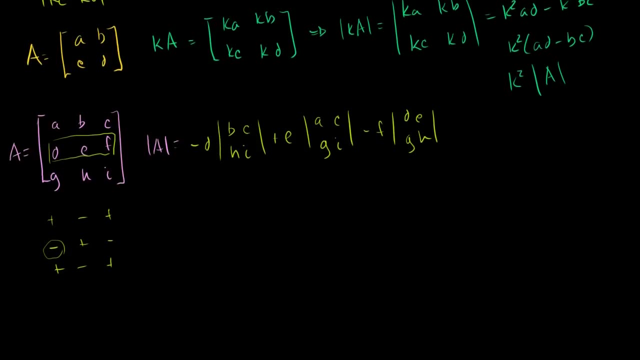 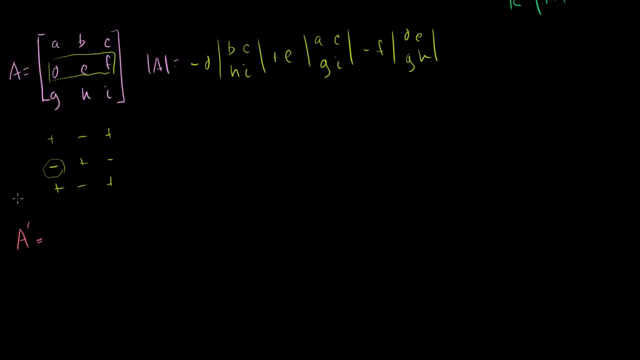 g, h. That's the determinant of this matrix A. Now what if we define some new matrix here? Let's call it A prime. Let me scroll down a little bit. Let me define A prime right here. A prime, I'm just going to multiply this row by a scalar. 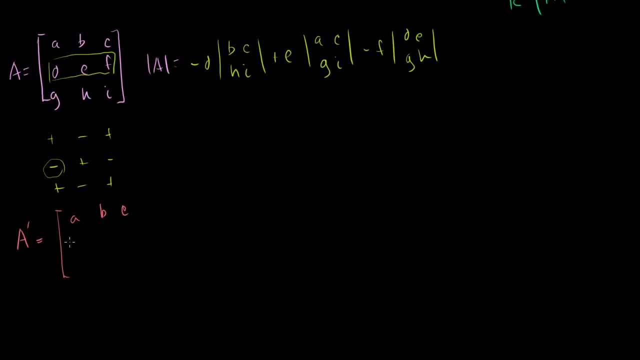 So it's going to be equal to a, b, c, k d, k e and k f. I'm not multiplying the whole matrix times the scalar. I can't say this is k a. I'm just multiplying one of its rows. 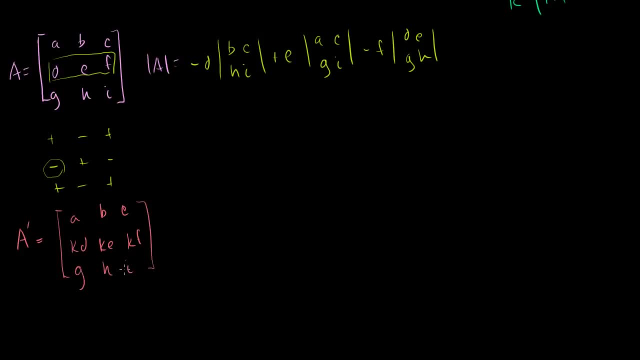 And then I have g, h and i. So what's the determinant of A prime going to be? And I put that prime there to show it's different than A, Or maybe it's, you know, but it's derived from A. 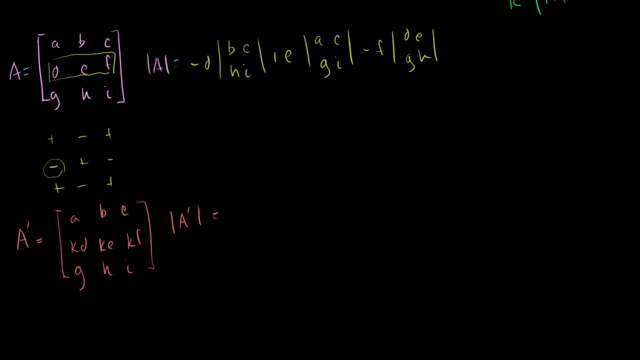 I just multiplied one row of A times the scalar. Well, I can go along that same row that I did up here. I go along that same row, And the only difference is that, instead of having a d, I now have a kd. 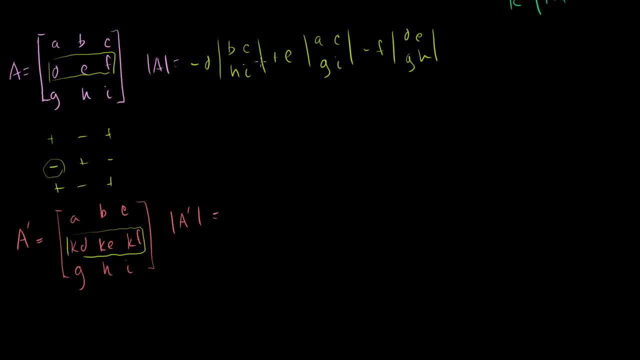 Instead of an e, I now have a ke. So instead of a d, I'm going to have a kd there. Instead of an e, I'm going to have a ke there. So it's going to be this exact same thing, but I can replace. 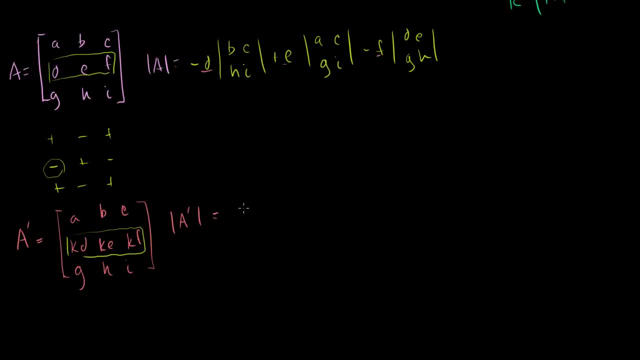 this guy, this guy and this guy with them multiplied by k, So it's going to be equal to minus kd times the determinant of the submatrix b, c, h, i. I'm not even going to look over here, because it's going to be. 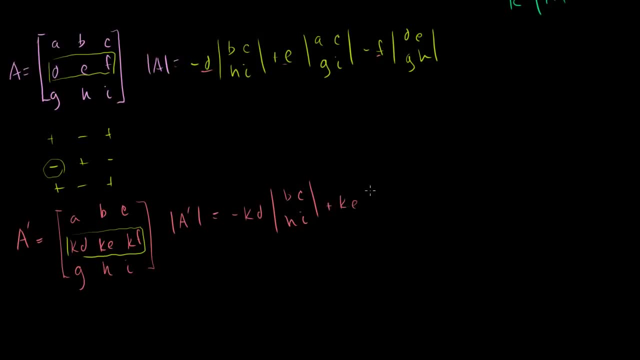 the same thing as that one up there, Plus ke times the determinant of A, c, g, i, plus minus, minus kd, kf times the determinant of d, e, g, h, And what is this equal to? This is equal to if you just factor out the k, it's equal. 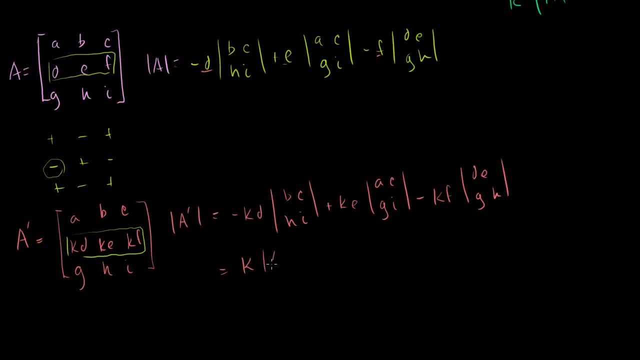 to k times this, So it's equal to k times the determinant of A. So our result also worked for the 3 by 3 case. I just happened to pick the middle row, but I encourage you to pick other rows and to see what happens. 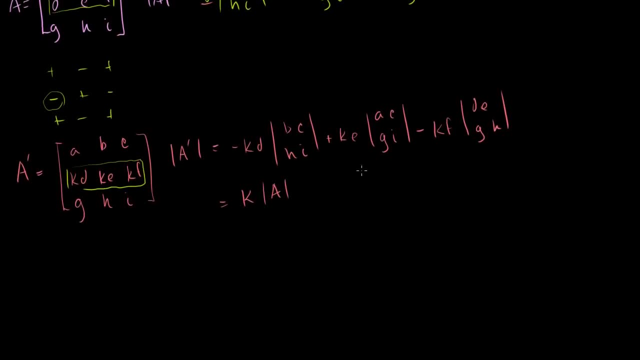 And so let's actually do it for the general case, because I've just been giving you particular examples And I'd like to show you the general proof when the general proof isn't too hairy. So let's say, I have an n by n matrix. 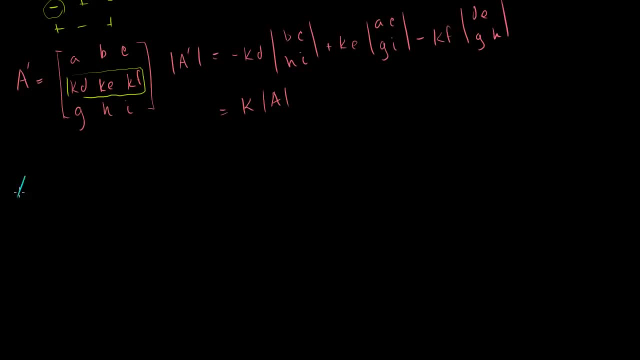 So let's say that I have a matrix A. Let's say that A is n by n, So it equals. you can write it like this: This is the first row, first column a11, a12, all the way to a1n. 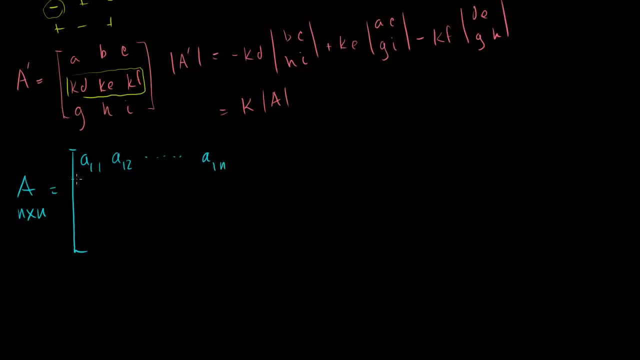 I'm going to pick some arbitrary row here that I'm going to end up multiplying by a scalar, So we could go down here: Let's say row ai, So this is ai, So this is ai, So this is ai1,, ai2,, all the way to ain. 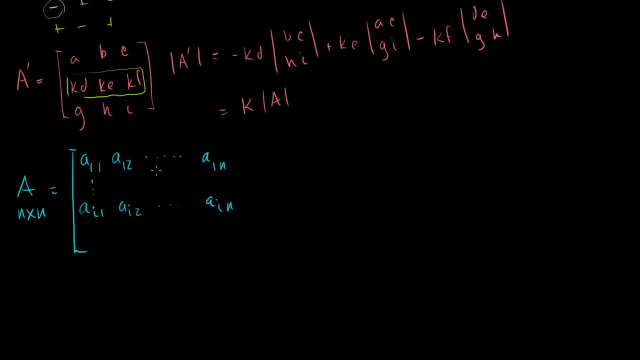 This is some row that I'm going to use to determine the determinant. Remember, we can go down any row to get the determinant. Then, finally, you keep going. You get an1,, an2,, all the way to ann. This is as general as you can get for an n by n matrix. 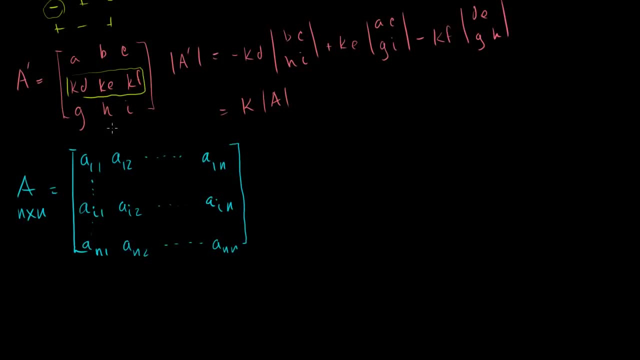 Now let's figure out its determinant. So the determinant of A- And I'm just going to go down this row right there- So the determinant of A is equal to what It's equal to. well, we have to remember the checkerboard. 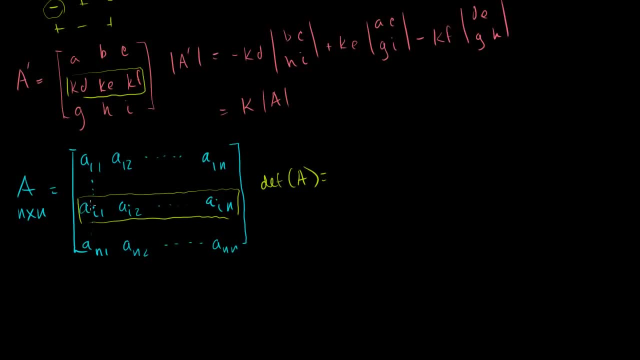 pattern and we don't know where we are in the checkerboard pattern because I just picked an arbitrary general row here. But we can use the general formula that the sine is going to be determined by negative 1 to the i. And you can use the general formula that the sine is going to be determined by negative 1 to the i. 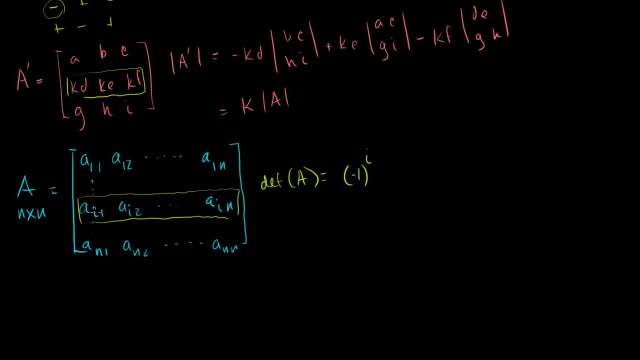 I don't know if i is even or odd, So it's going to be. i plus for this term, 1 power. That's its sine. This is what gives us the checkerboard pattern. Let me make that clear because it looks complicated. 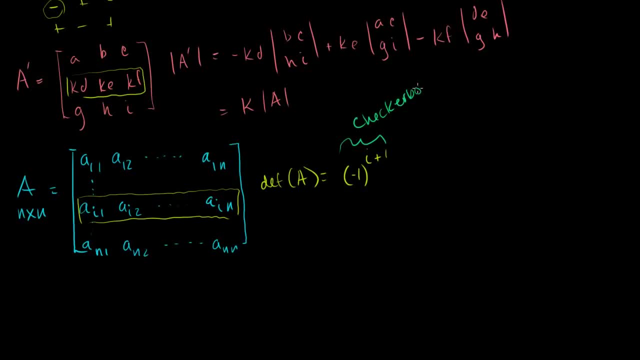 But this is just the checkerboard pattern, That's just that. right there. Times this term. right there. So times ai, so the coefficient ai1.. And then times this guy's submatrix, And you remember the submatrix. You get rid of this row and this column. 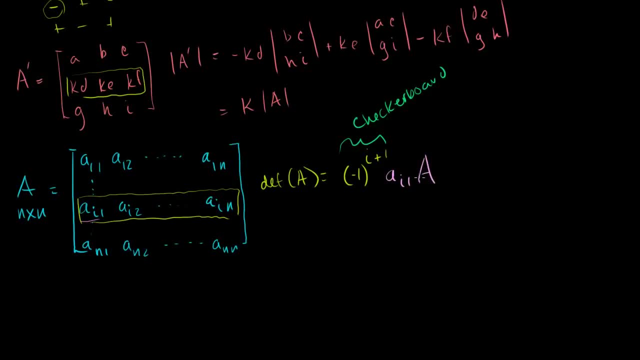 It's going to be everything that's left over, So times that submatrix of ai1.. And then you're going to keep and it's going to be plus- let me just keep doing it- plus negative 1 to the i, plus 2. 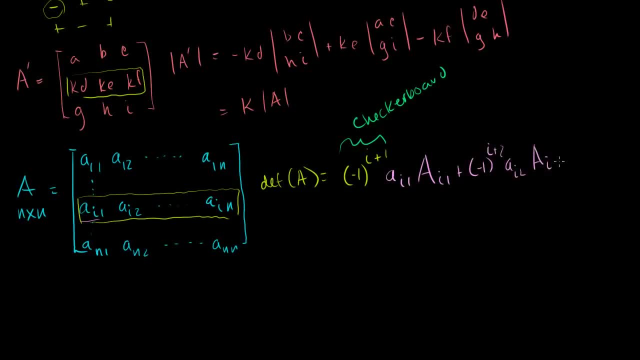 times ai2 times its submatrix i2.. All the way you just keep going. plus minus 1 to the i plus n. Okay, Plus n times ai, you're in the nth column, And then its submatrix. This is going to be an n minus 1 by n minus 1 matrix. 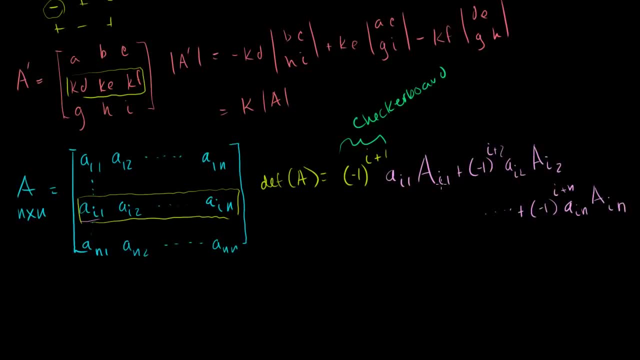 All of these are going to be in Just like that. That's the determinant of A, And we could actually rewrite it in sigma notation. That'll simplify things a little bit. So the determinant of A, we can rewrite it as the sum from j. 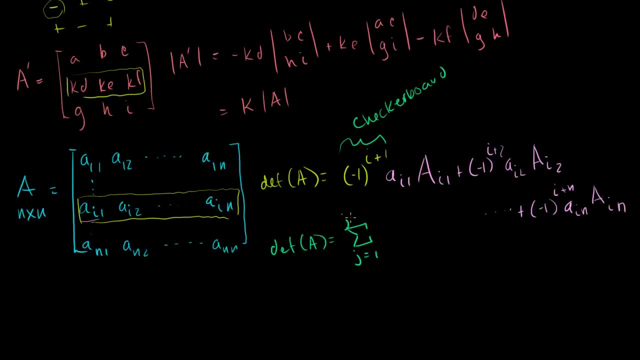 is equal to 1 to j. I'll write it explicitly here: j is equal to n Of negative 1 to the i plus j times aij and then each of the submatrices aij. This thing right here is just another way of writing this. 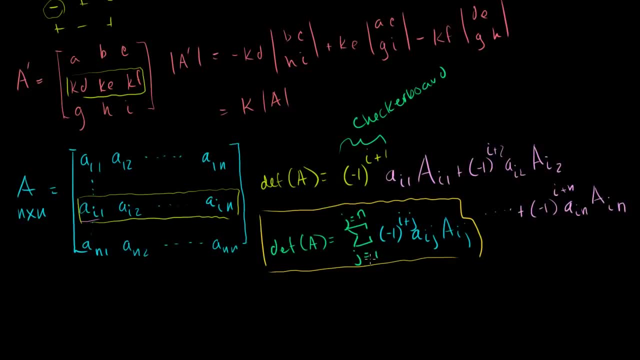 thing I wrote up there. I'm just saying the sum, You just take j equal 1, put them in there, you get this term right there. You take j equal 2.. You add it, you get this term right there. 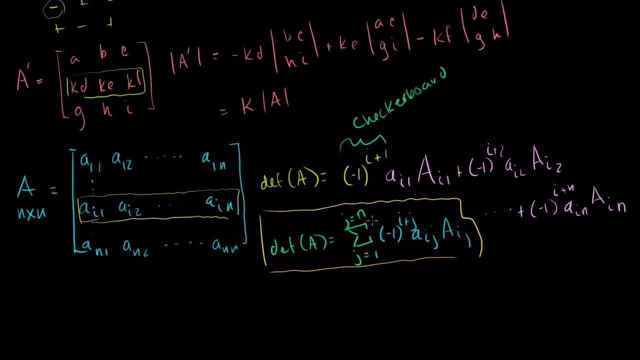 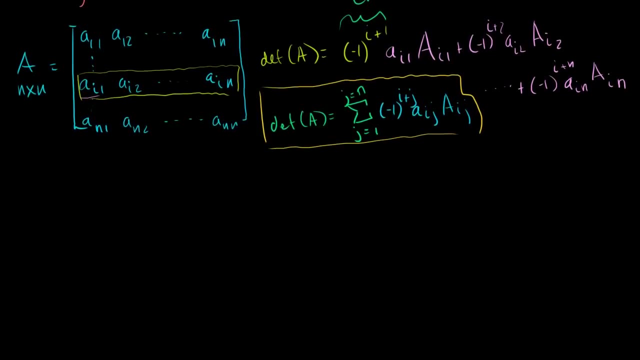 You keep doing it, you get j equal n. You get that term right there. So these two things are equivalent. So what happens if I have some new matrix? Let's say, let me copy and paste my current matrix. So let me copy and paste it. 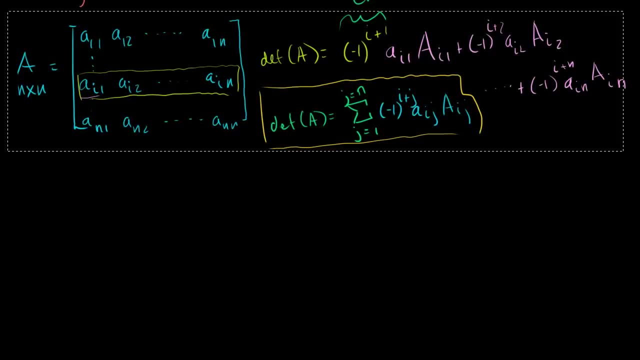 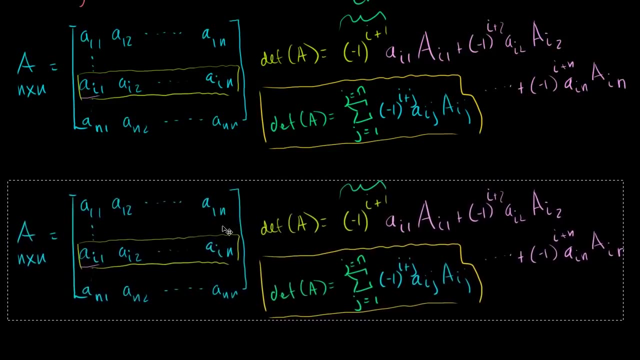 Actually, let me copy and paste everything. Let me copy and paste everything. That'll make things move quickly. I copied it and now let me paste it, just like that. And let me define a new matrix. Let me define my new matrix: a prime. 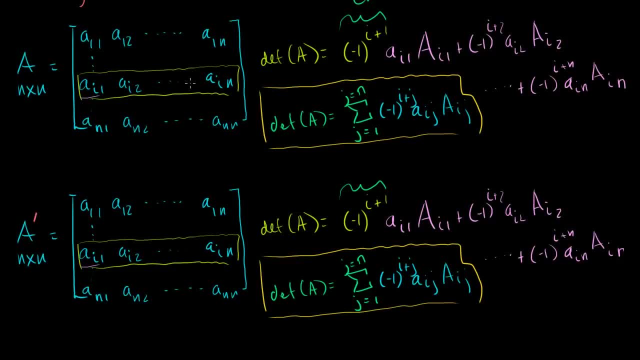 It's still an n by n matrix, but that row that I just happened to use to determine my determinant, I'm going to multiply it by a scalar k, So it's kai, ka1, kai2, kain, just like that. 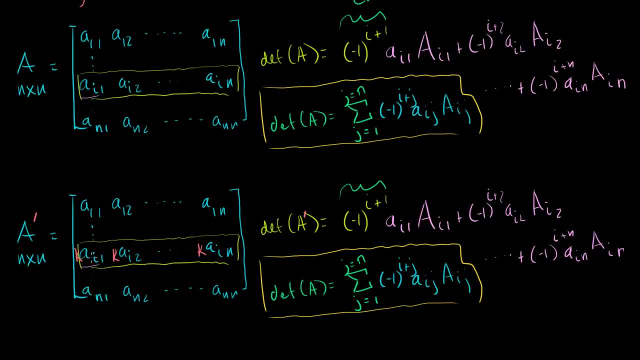 So what's the determinant of a prime? Well, we're just going to go down this row again, But now, instead of just an ai1, we have a kai1. instead of an aij Right 2,, we have a kai 2.. 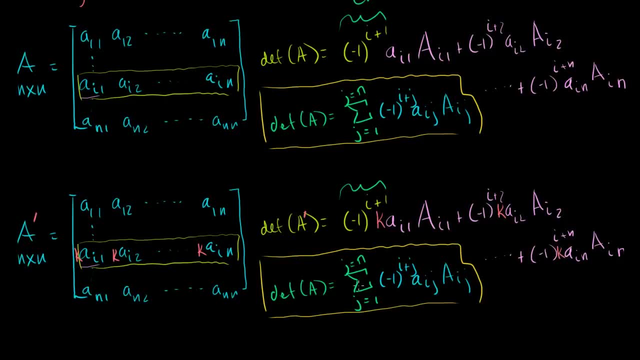 Instead of a kain, we have a kain, So its determinant is just going to be this same thing. but instead of an aij, everywhere we're going to have a kaij, So this is going to be the determinant of a prime. 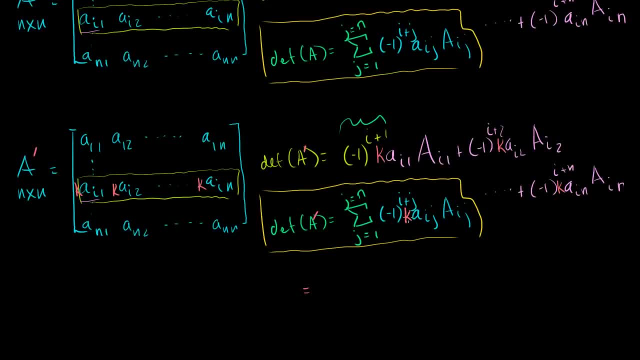 And so this is equal to. we could just take out this constant right here. It has no i's or j's in it, so it has no j's in it in particular, so we can just take it out. So it's equal to k times the sum from j is equal to 1 to j. 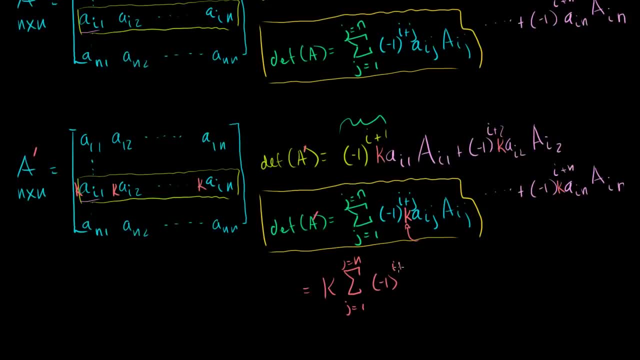 is equal to n of minus 1, to the i plus j times aij, and this is the coefficient. and then this is the submatrix for each of those coefficients: aij, that's a matrix right there, an n minus 1 by n minus 1 matrix. 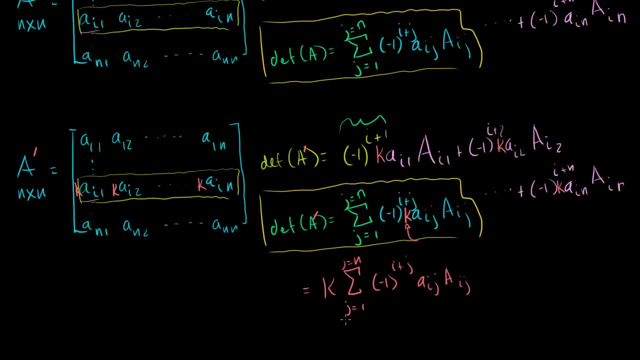 And then you know, you immediately recognize. I think you saw where this was going. This right here is just the determinant of a kaij. So we get the result that the determinant of a prime is equal to k times the determinant of a. 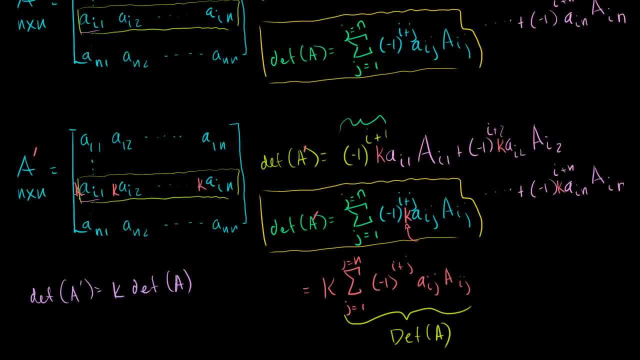 So we've just shown you in general, you have any n by n matrix. If you multiply only one row, not the whole matrix, only one row, by some scalar multiple k, the resulting determinant will be your original determinant times k. Now 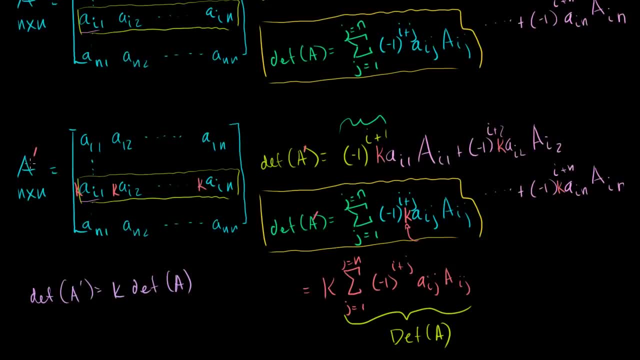 I touched on this in the original video. What happens if you keep? what if you multiply? what is the determinant? what is the determinant of k times a? So now we're multiplying every row times k, Or another way to think about it is: you're multiplying I. 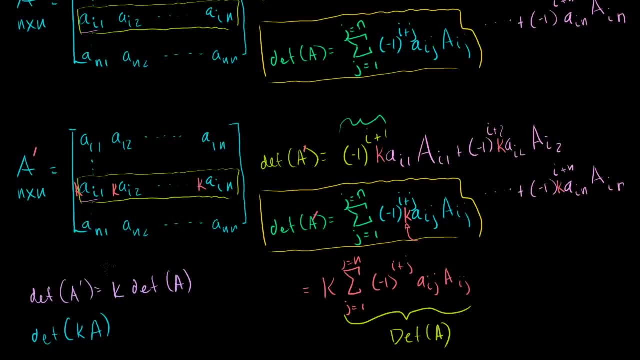 guess you're multiplying n rows times k, right? So you're doing this n times. So if you multiply k times itself n times, what do you get? You get k to the n, So this is going to be equal to k times a. 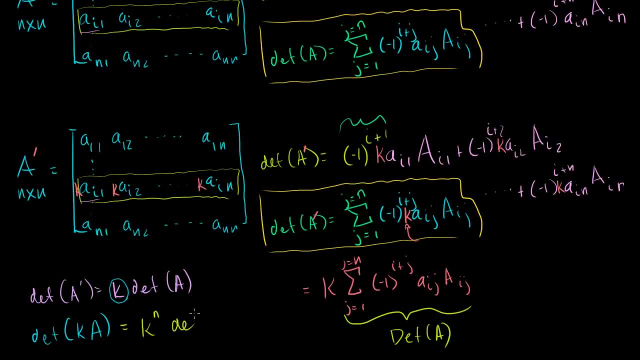 Equal to k to the n times the determinant of a Right. If you just do it once, you get k times the determinant of a. Now, if you do a second row, you're going to get k times k times the determinant of a. 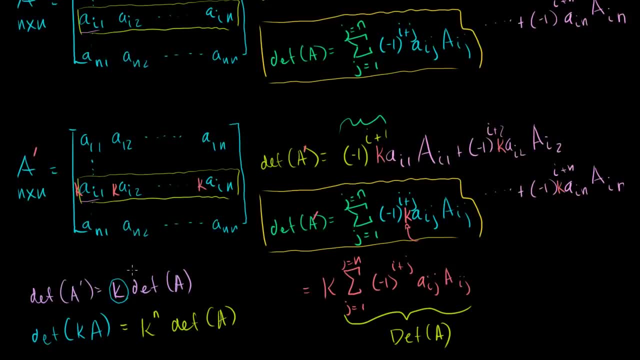 You do a third row, you're going to get k to the third times the determinant of a. The fourth row, k to the fourth times the determinant of a. If you do them all, all n rows, you're going to have k to the. 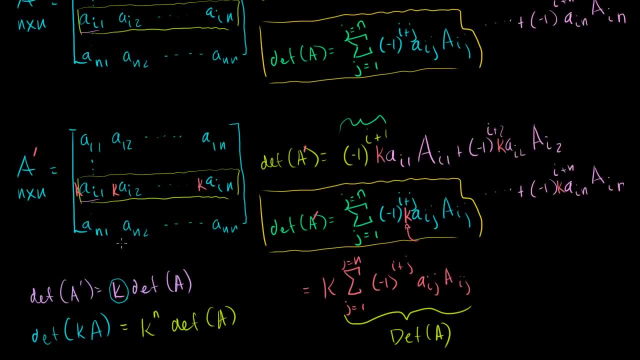 n times the determinant of a. Anyway, hopefully you found that interesting And I encourage you to experiment with this other ways, Try going down a column and seeing what happens.